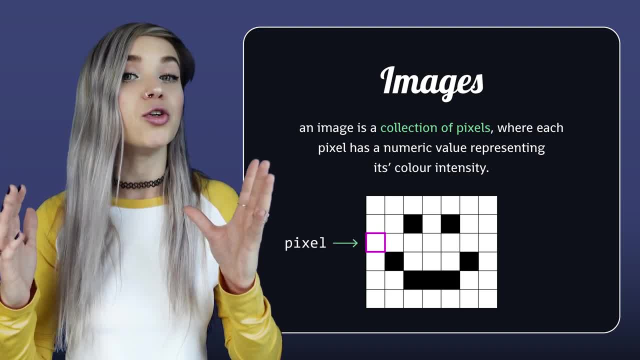 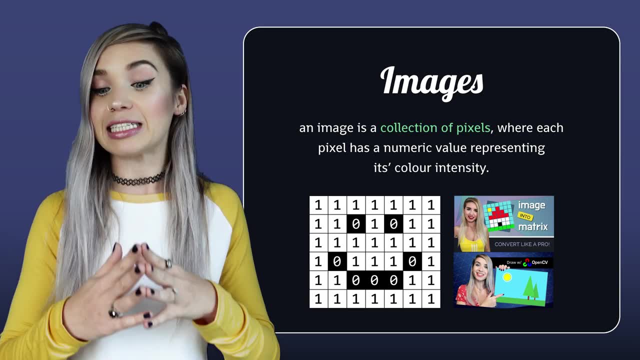 And in both cases we have a brain power. we don't understand. When a computer sees its image, it of pixels, where each pixel stores a numeric value representing the color intensity. We already talked about it in previous lessons and you guys can definitely check it out, if you haven't. So then, instead of a goat photo, our 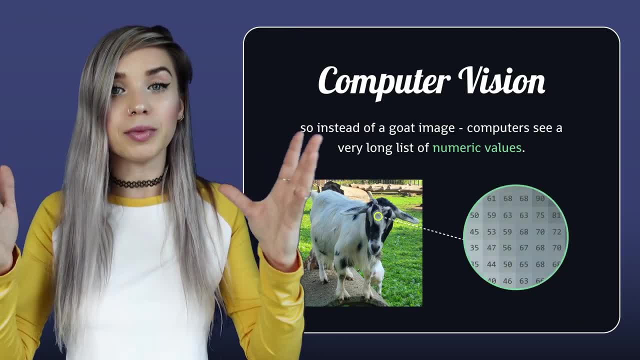 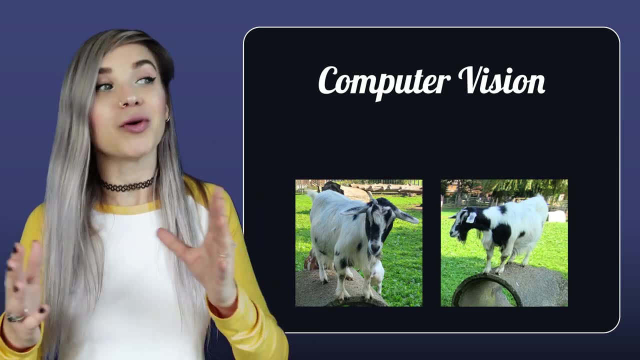 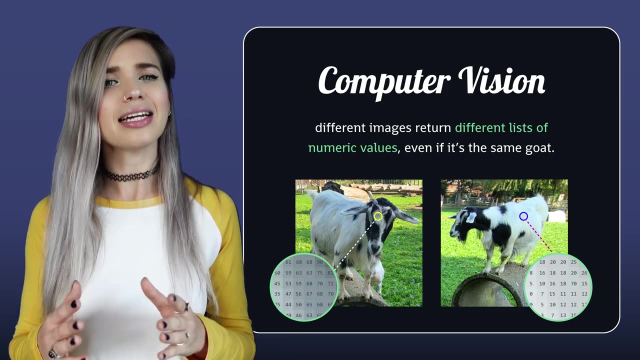 computer sees a very long array of numeric values. And then the tricky part is: even if we take another photo of the exact same goat on the exact same background, we will most likely get a brand new array of numeric values. And guess what? Even if we use the original photo but slightly boost the brightness. 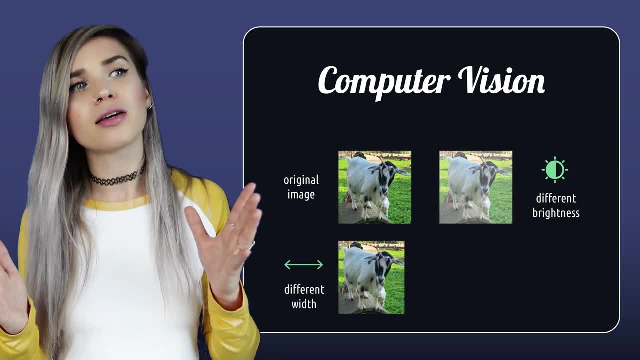 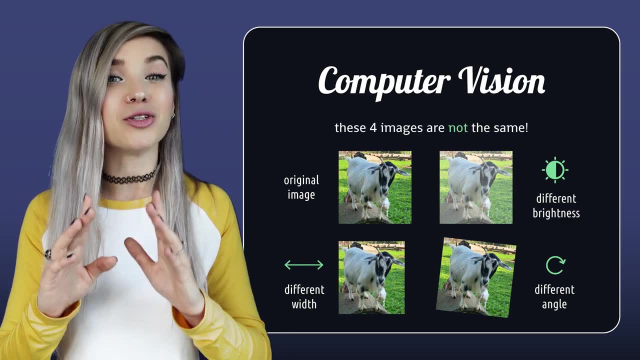 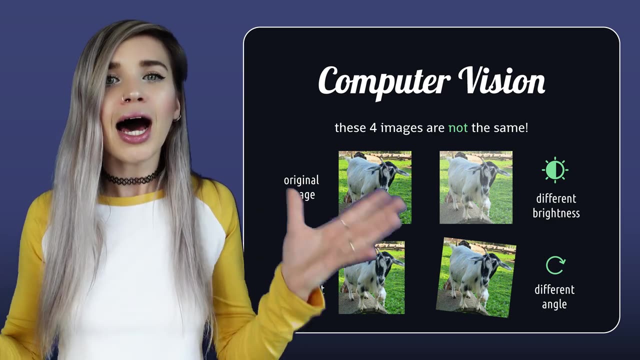 or maybe crop five pixels from the width, or even just rotate it five degrees clockwise, we still get a brand new array of numeric values that has nothing to do with the original one. So if it is so difficult, how can we ever classify an image and left alone recognize a face in it? We simply expose. 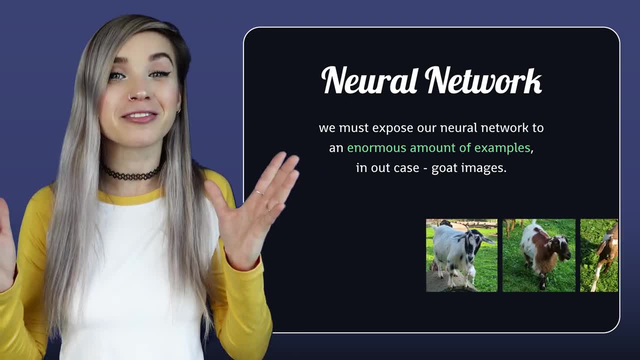 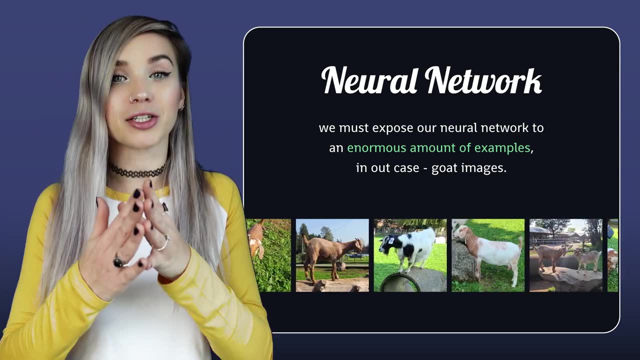 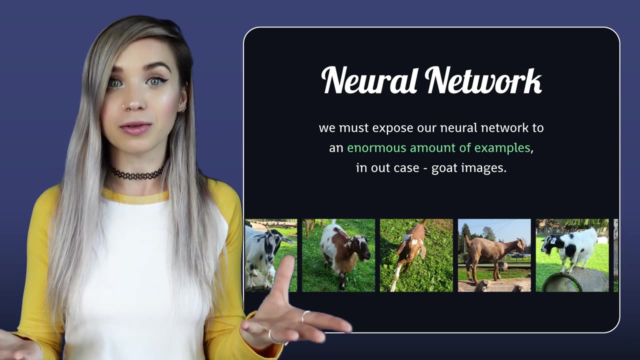 our neural network to an enormous amount of images. Each image is an example, and the more examples we provide, the bigger the chance that our neural network recognizes the subject. In our case, that would be the class or category of goat. But that's not all. Our examples also need to be interpreted properly. 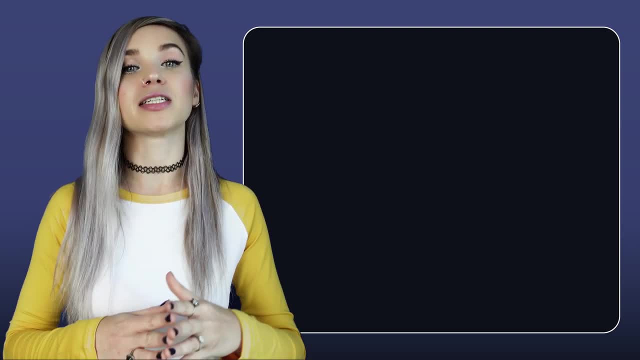 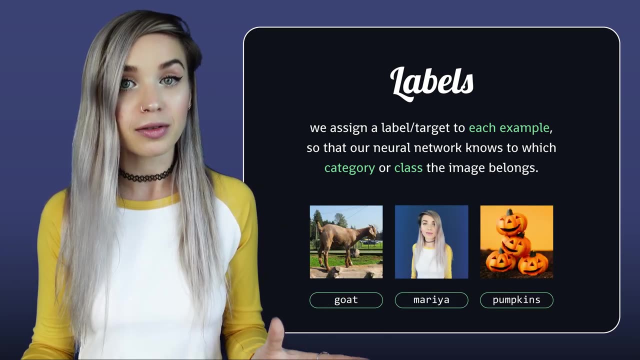 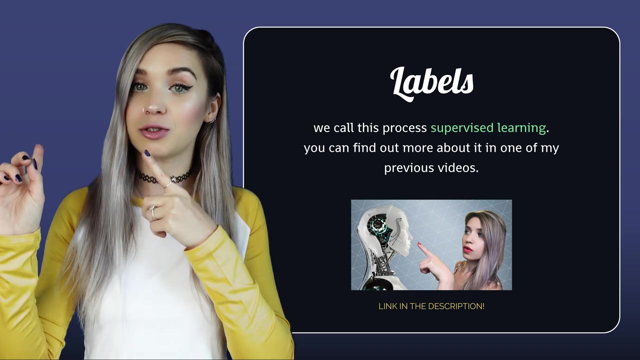 That's why, very often, each example will have something called a label or a target that tells our neural network to which category it belongs. We call this process supervised learning, and if you guys want to find out more about it, you can check out my previous tutorial. But between the point, 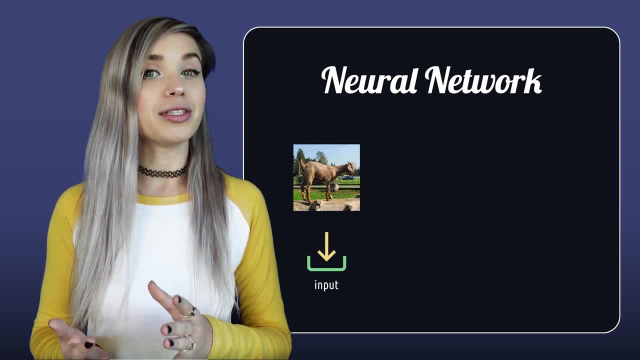 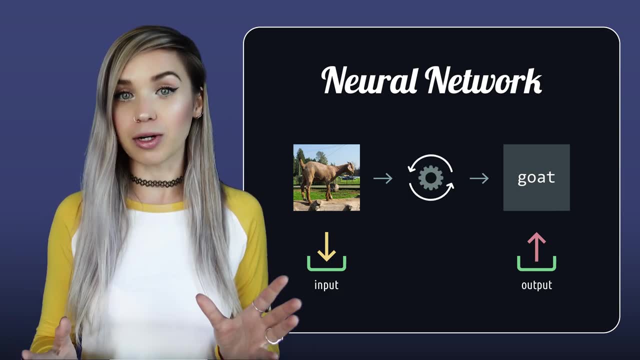 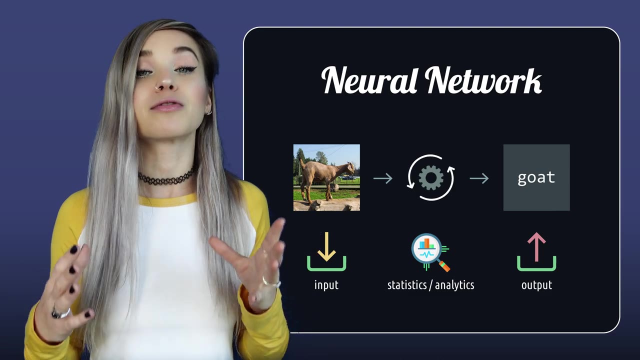 where we feed an image to our neural network and the point where we reach the conclusion that it's a goat. a lot of different processes are happening in the background. These are series of statistical calculations that investigate each of our examples from many different angles. These calculations happen inside something called 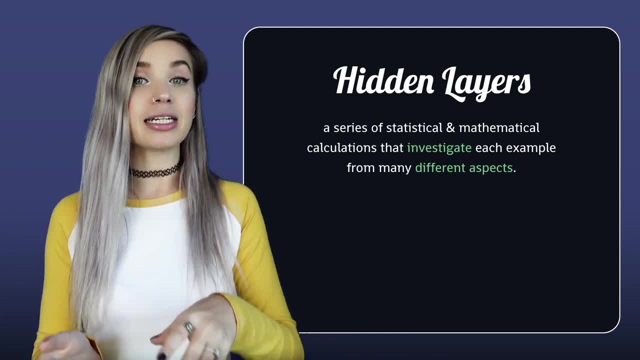 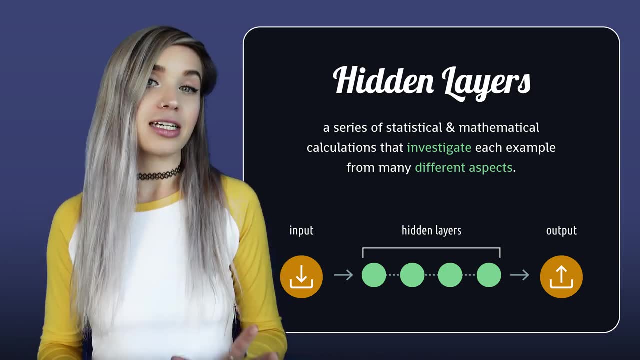 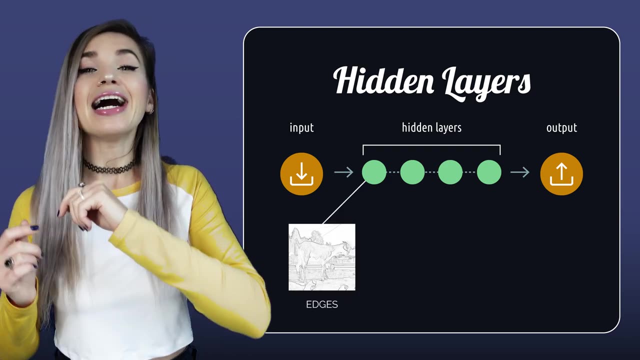 hidden layers. They are located in between our input layer and our output layer and they are responsible for evaluating different aspects of our examples. For example, one hidden layer is responsible for edge detection, another hidden layer maps the colors, another one counts the legs. 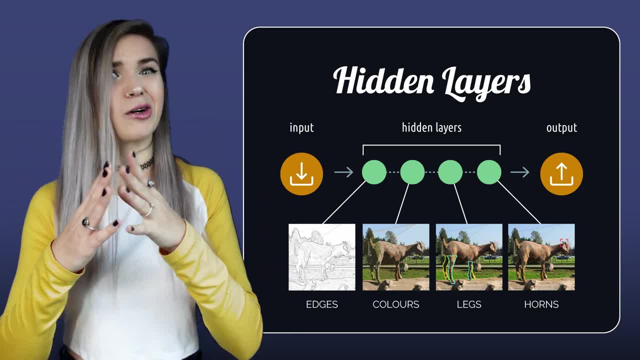 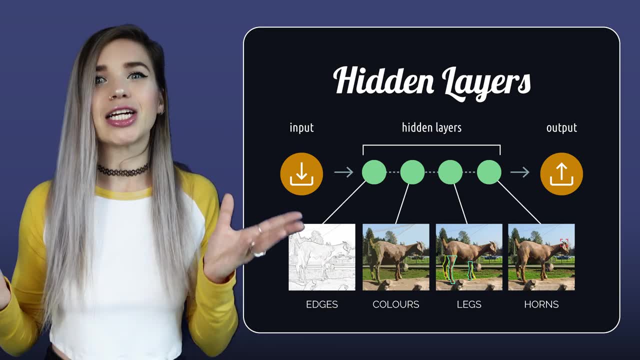 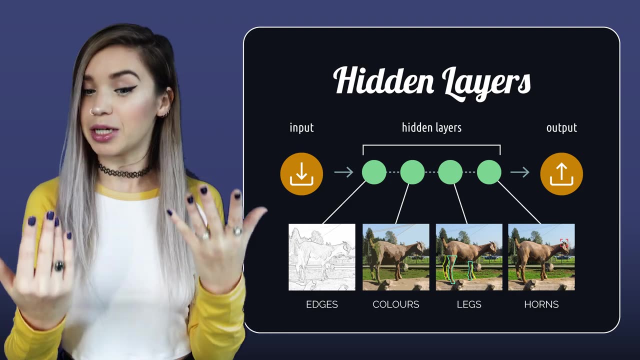 or maybe even detects horns. Now, on their own these layers are quite useless. Just because something has horns doesn't really make it a goat. But when we combine all these layers together, we actually have enough information to make a prediction. So an image is loaded into the input. 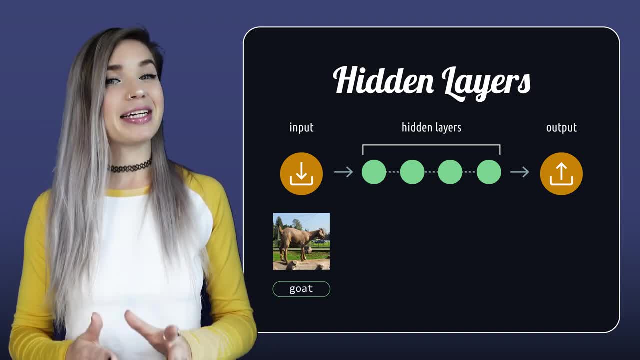 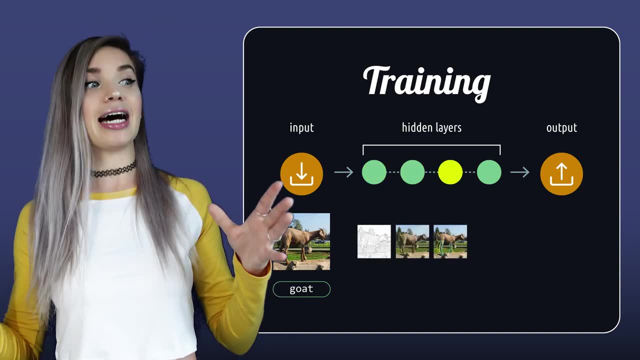 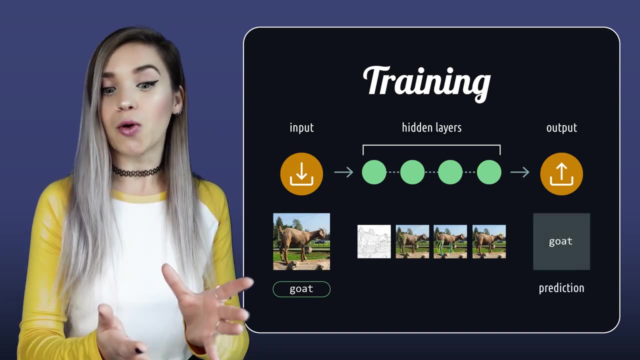 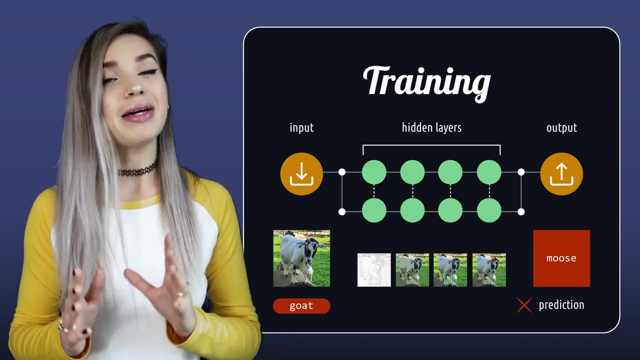 layer, along with its label. This is where we begin training our neural network. The image will then pass through each of our hidden layers, one at a time, and once we reach the output layer, our network will return a class name, which we call a prediction. This class name, however, will not always match the label, and the main reason are: 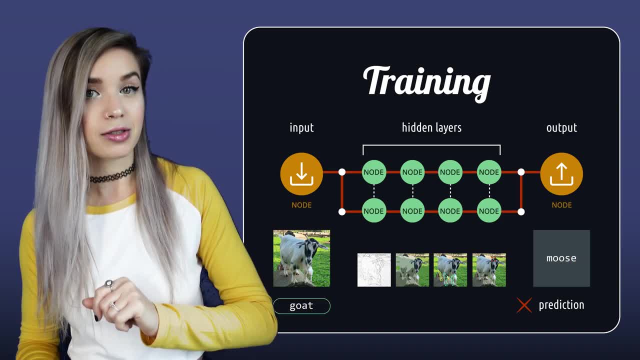 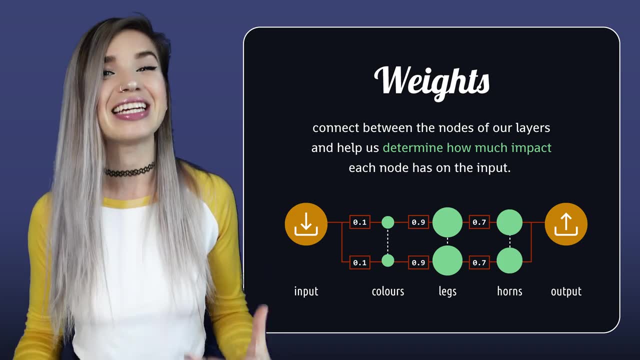 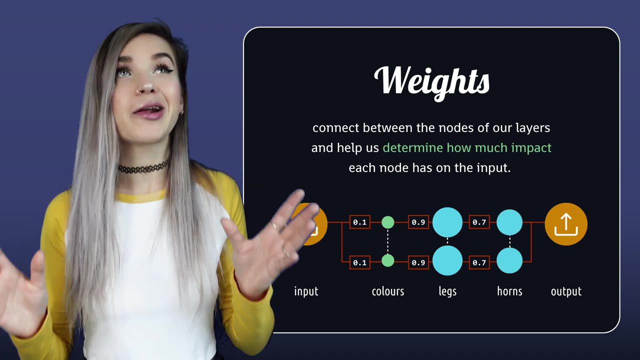 those links that connect between the nodes of our layers. We call these links weights, and they help determine how much impact each node has on the input. For example, maybe counting legs or detecting horns is much more meaningful than mapping colors. In that case, the weights that lead to the color 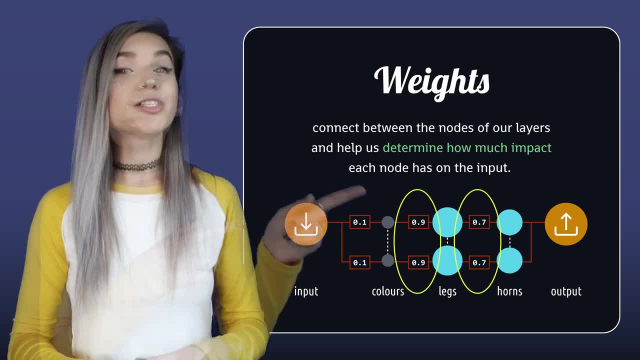 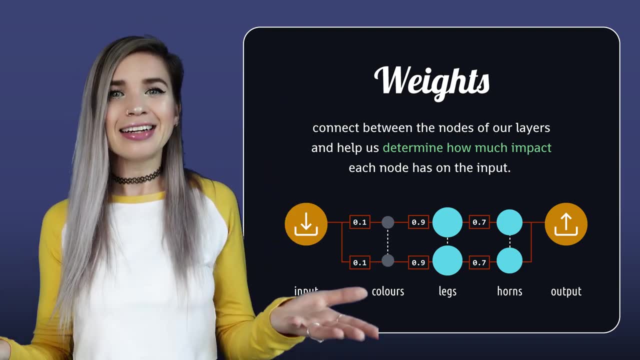 layer will have lower values than the other two. So just because our first prediction is incorrect, it doesn't mean that our neural network is bad. It only means that we need to keep adjusting the weights to match the values of each node, And that's why we call these links weights, and they help. 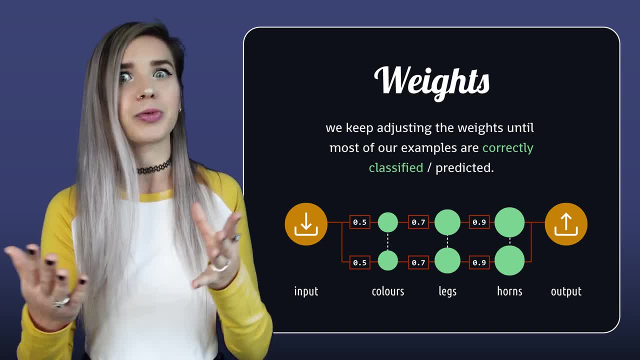 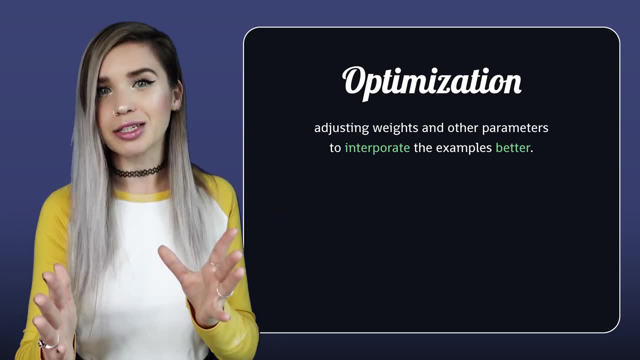 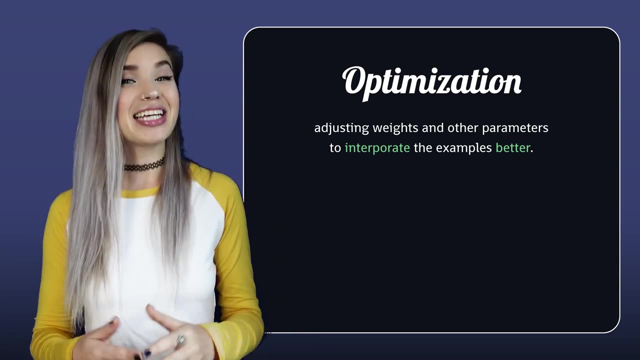 until most of our examples are correctly classified or predicted. We call this process optimization. It can take a very long time and we would usually optimize other parameters as well, not just the weights, but we'll talk about it in future lessons. But the good news are, once we are done optimizing